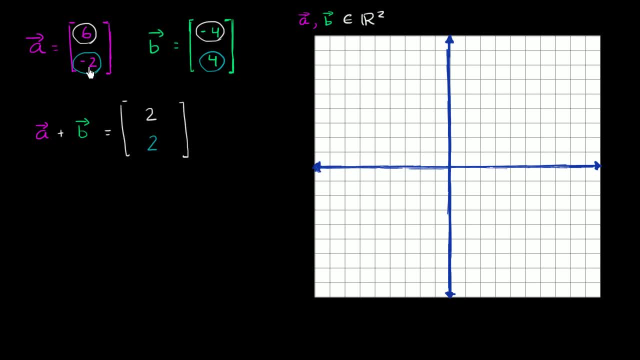 So vector a we could visualize. This tells us how far this vector moves in each of these directions: Horizontal direction and vertical direction. So if we put the- I guess you could say the tail of the vector- at the origin. Remember, we don't have to put the tail at the origin. 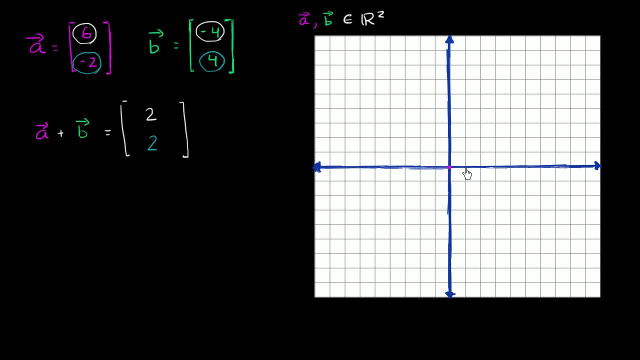 but that might make it a little bit easier for us to draw it. We'll go six in the horizontal direction: One, two, three, four, five, six, And then negative two is the second one. Negative two in the vertical, so negative two. 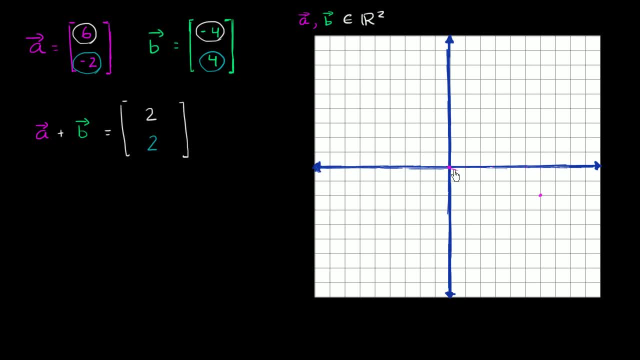 So vector a could look like this, Vector a looks like that And, once again, the important thing is the magnitude and the direction. The magnitude is represented by the length of this vector and the direction is the direction that it's pointed in. 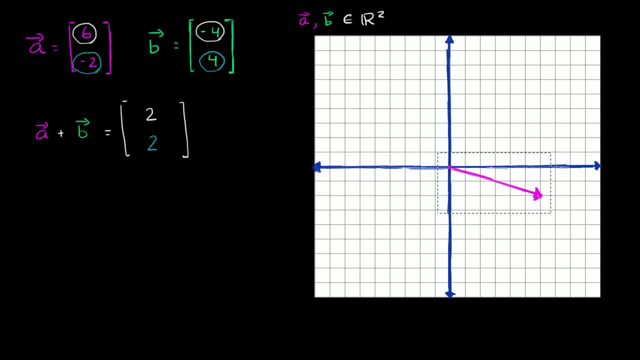 And also just to emphasize, I could have drawn vector a like that, or I could have put it over here. These are all. These are all equivalent vectors. These are all equal to vector a. All I really care about is the magnitude and the direction. 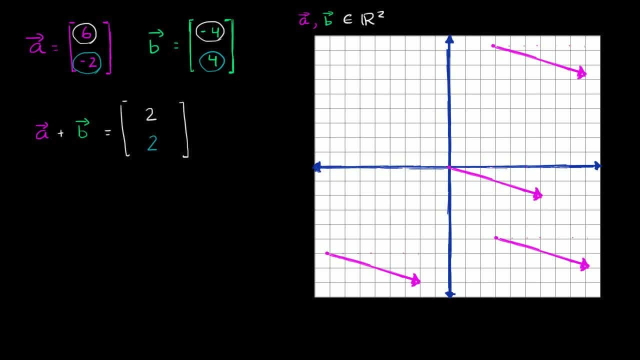 So with that in mind, let's also draw vector b. Vector b, in the horizontal direction, goes negative: four, One, two, three, four. And in the vertical direction it goes four, One, two, three, four. So its tail, if we start at the origin. 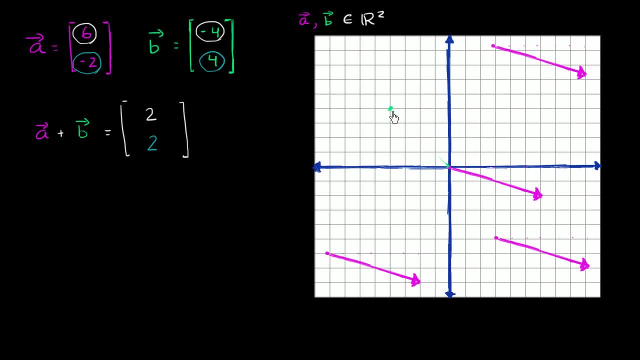 if its tail is at the origin, its head would be at four, it would be at negative 4, 4.. So let me draw that just like that, So that right over here is vector b And once again vector b. we could draw it like that. 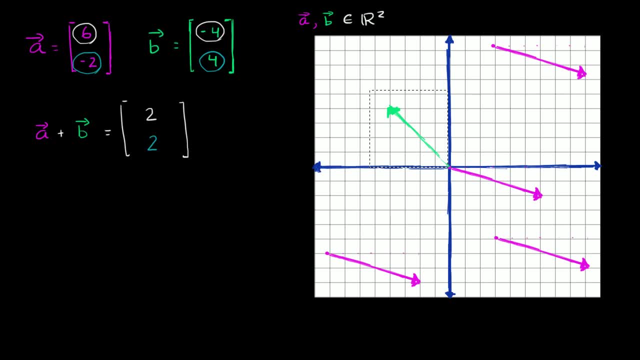 or we could draw it. so let me copy, let me paste it. So this would also be another way to draw vector b. This would also be another way to draw vector b. Once again, what I really care about is its magnitude and its direction. 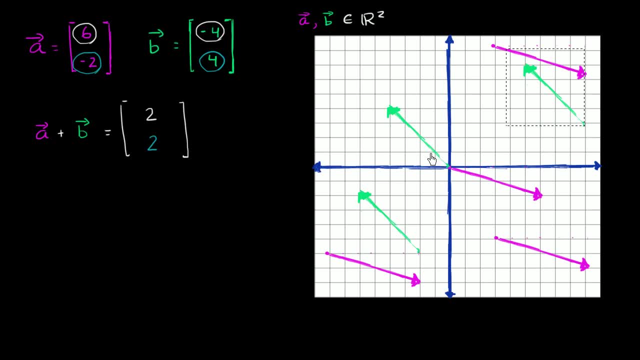 All of these green vectors have the same Magnitude, they all have the same length and they all have the same direction. So how does the way that I drew vector a and b gel with what its sum is? So let me draw its sum like this: 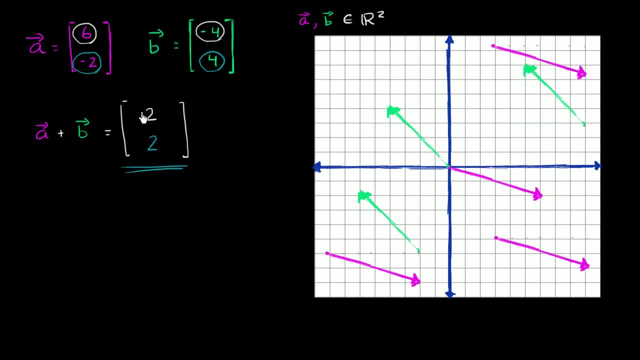 Let me draw its sum in this blue color. So the sum based on this definition- we just used a vector addition- would be 2, 2.. So 2, 2.. So it would look something like this: So how does this make sense that the sum 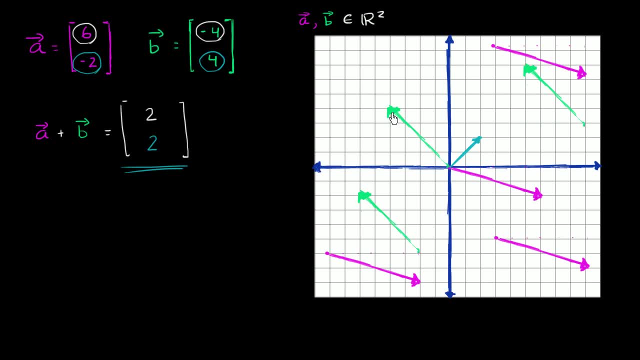 that this purple vector would look like this. So the sum of this purple vector plus this green vector is somehow going to be equal to this blue vector. I encourage you to pause the video and think about if that even makes sense. Well, one way to think about it is this first purple vector. 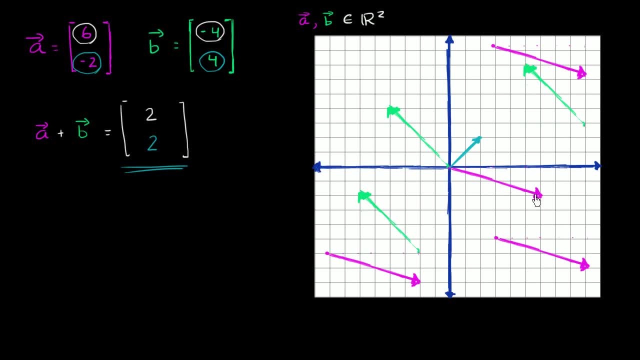 it shifts us this much. It takes us from this point to that point, And so, if we were to add it, let's start at this point and put the green vector's tail right there and see where it ends up putting us. So, the green vector, we already have a version. 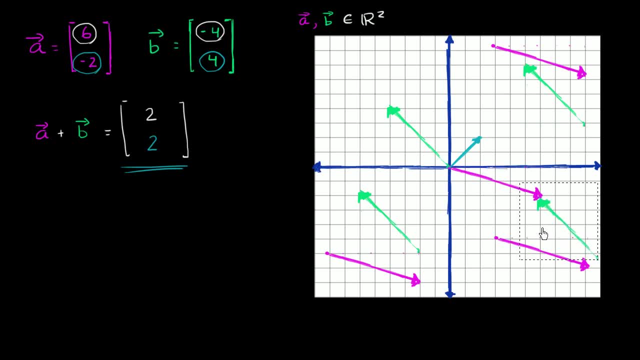 So once again we start The origin. the vector a takes us there. Now let's start over there with the green vector and see where green vector takes us. And this makes sense: Vector a plus vector b. Put the tail of vector b at the head of vector a. 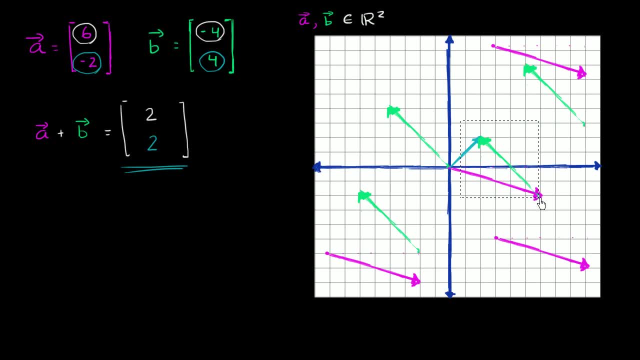 So if you were to start at the origin, vector a takes you there. Then if you add on what vector b takes you, it takes you right over there. So, relative to the origin, how much did you? I guess you could say shift? 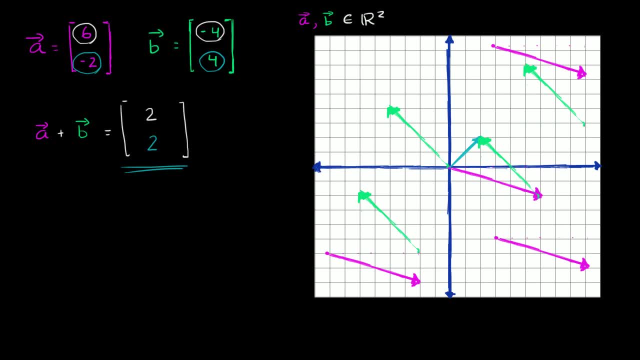 And once again, vectors don't only apply to things like displacement, They apply to velocity, It can apply to actual acceleration, It can apply to a whole series of things, But when you visualize it this way, you see that it does make complete sense. 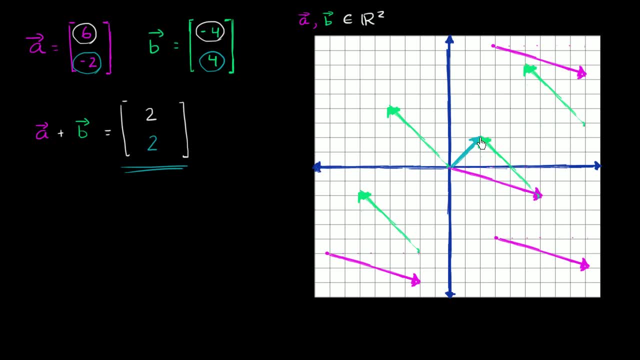 This blue vector. the sum of the two is what results. where you start with vector a. At that point, right over there, vector a takes you there. Then you take vector b's tail, start over there and it takes you to the tip of the sum. 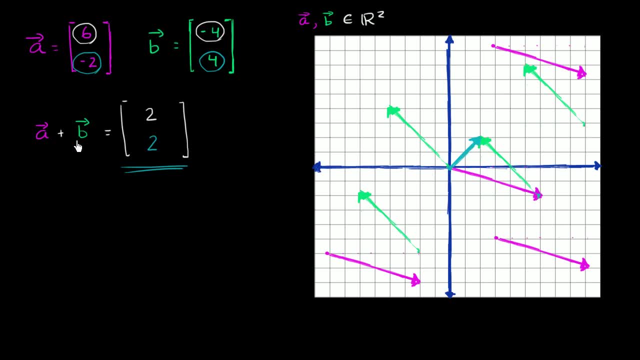 Now one question you might be having is: well, vector a plus vector b is this, but what is vector b? What is vector b plus vector a Plus vector a? Does this still work Well, based on the definition we had? 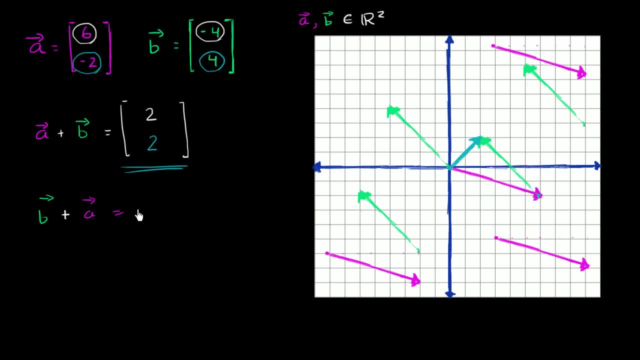 where you add the corresponding components, you're still going to get the same sum vector, So it should come out the same. So this will just be negative. 4 plus 6 is 2.. 4 plus negative 2 is 2..